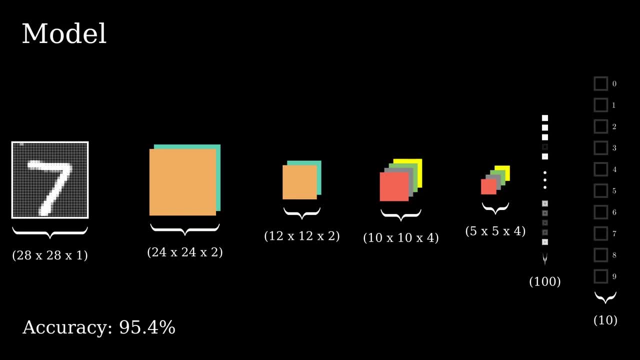 Now let's have a look at all the layers. Before we start, We'll input images from the mNIST dataset. This is a dataset consisting of handwritten digits from 0 to 9.. After inputting the image, we will perform a convolution. We'll 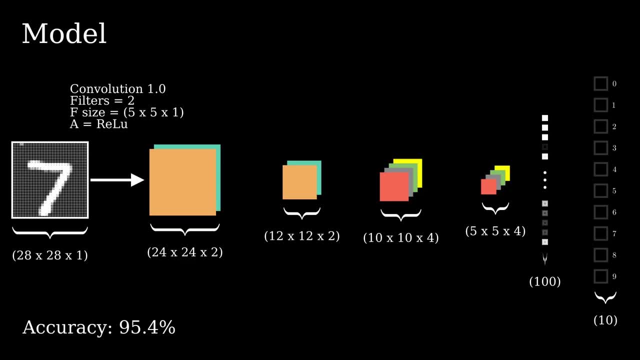 use two filters, or kernels as they're called, that have the dimensions 5 by 5 by 1.. The activation function denoted as A is ReLU. Next we'll perform max pooling with a pool size of 2 by 2 and 5 by 1.. Next we'll perform max pooling with a pool size of 2 by 2 and 5 by 2, and then. 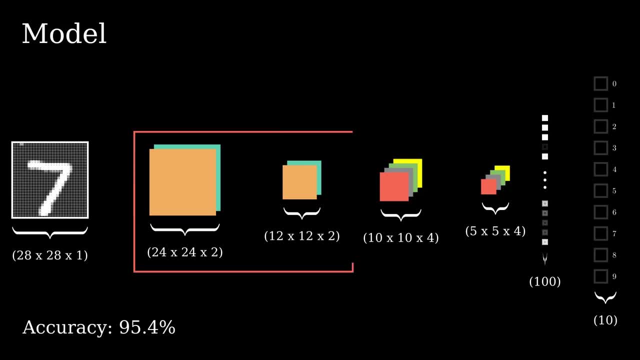 we'll perform max pooling with a pool size of 2 by 2 and 5 by 1, and then we'll perform max pooling 2 and a stride of 2.. This is our first layer. Then we move on by performing our second convolution. 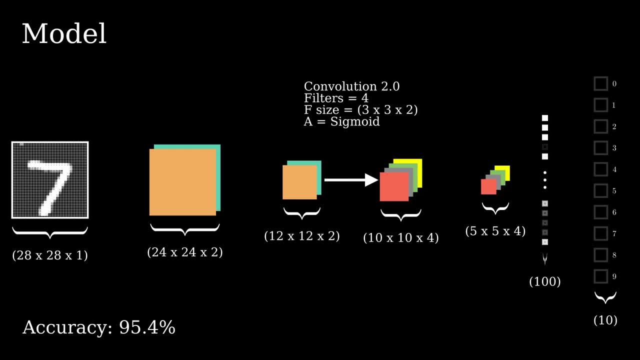 This time we'll use four filters that have the dimensions 3x3x2.. The activation is sigmoid. We'll then perform max pooling, exactly as earlier, before we flatten the matrices out. This gives us a flattened layer with 100 nodes. Here is our second layer. Finally, we have a fully connected 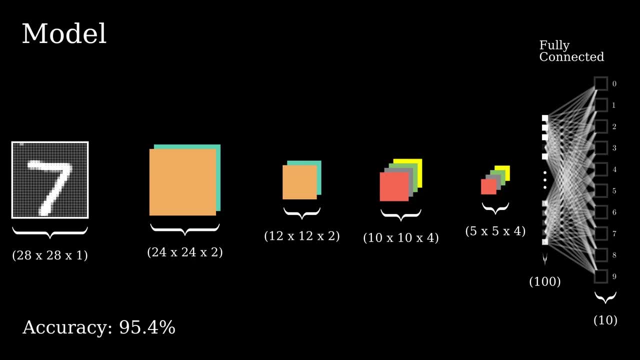 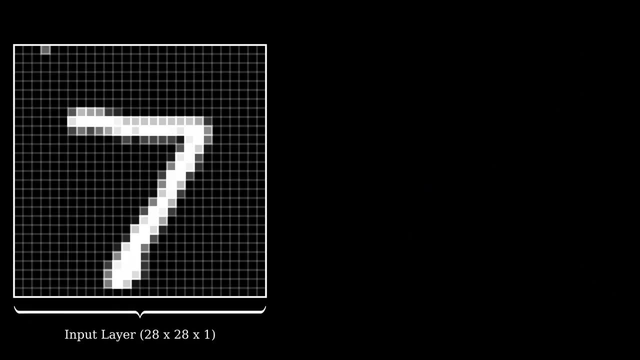 dense layer which outputs our predictions. Without wasting any more time, let's see the model in action. We start with the input layer, which is a 28x28x1 dimensional grayscale image. The image is fed into the first convolutional layer that consists of two 5x5x1. 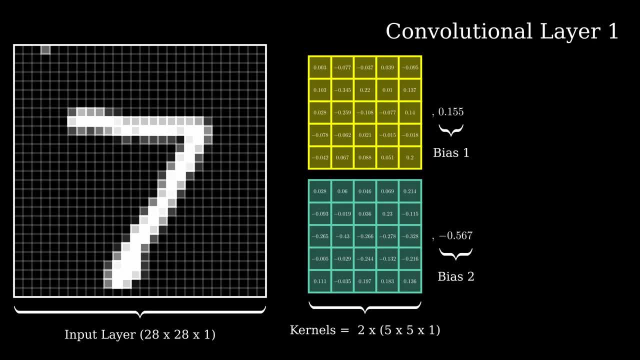 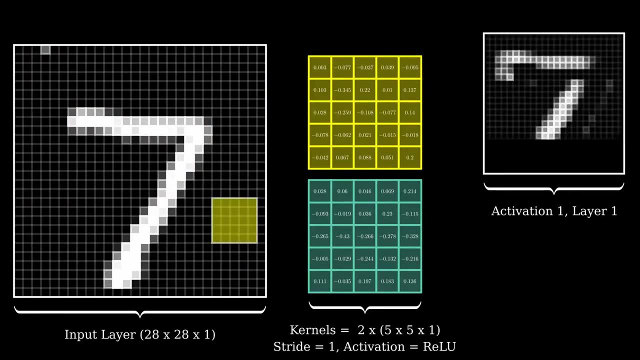 dimensional filters and two biases. One for each filter We'll use a stride of 1 and an activation function called ReLU. We start with the first filter and map the activations onto activation 1 in the first layer. Then we do the exact same thing for the second filter. 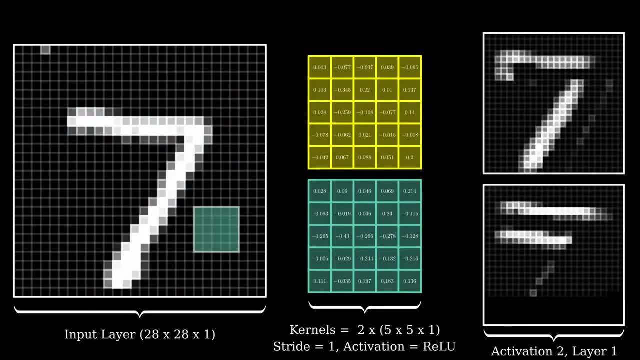 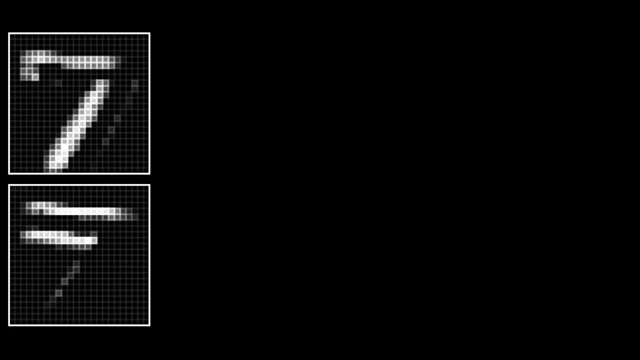 and map the output onto activation 2 in the first layer and move on. As you can see, the first convolution outputs two different images or matrices. These are called channels. Next up is the max pooling. We'll use a pool size of 2x2 and a. 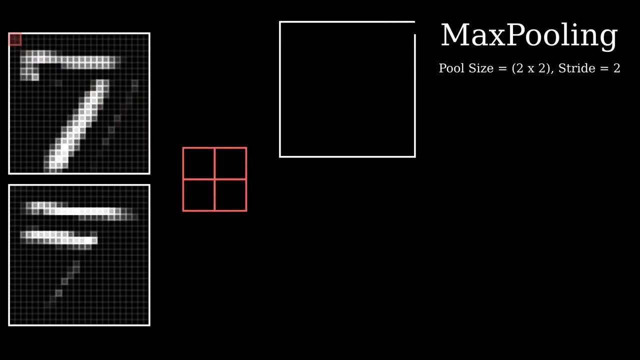 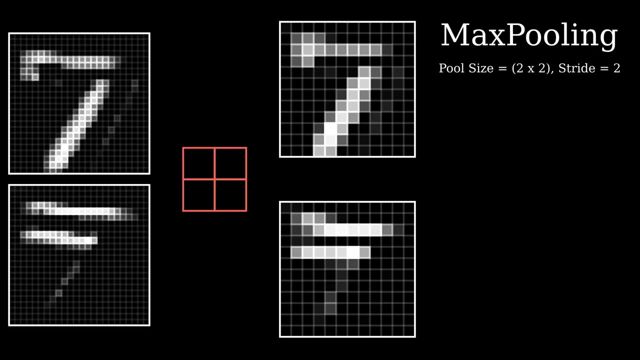 stride of 2.. We run the pooling for each of the channels and output them respectively. The idea is that we want to extract only the most activated pixels from the first convolution and shrink the dimensions. As you can see, we have shrunk the dimensions. 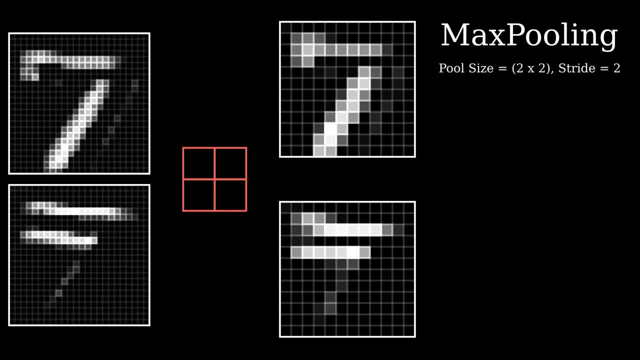 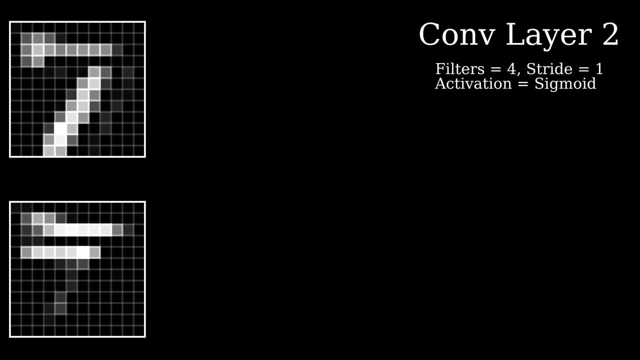 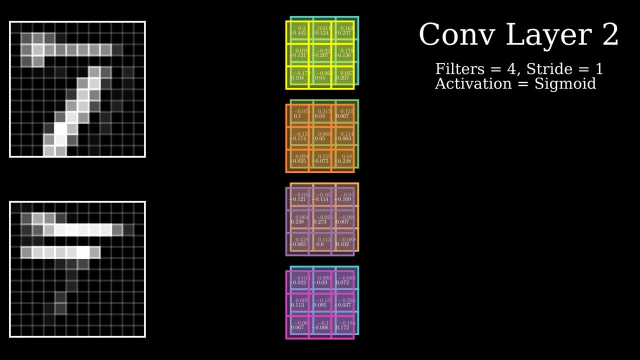 from 24x24x2 into 12x12x2.. Have a go and count the pixels if you'd like to. Next is the second convolutional layer. Here we'll use four filters with a stride of 1 and an activation function called sigmoid. As you probably noticed by now, these filters are stacked. 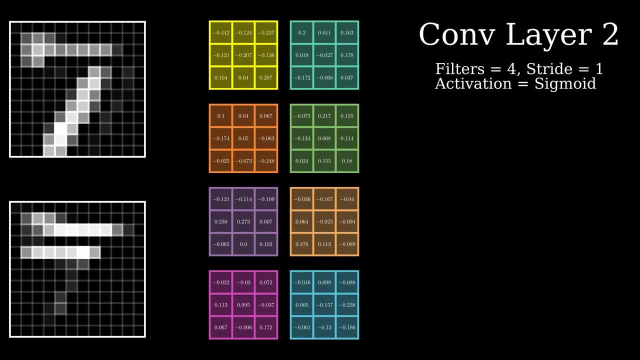 If we separate them, you'll see that we actually have eight filters. So what's going on? Well, there are four filters with the dimensions 3x3x2.. Since we have two channels from the previous activations, we'll have two channels in each filter. In addition, we also have one bias for each filter. 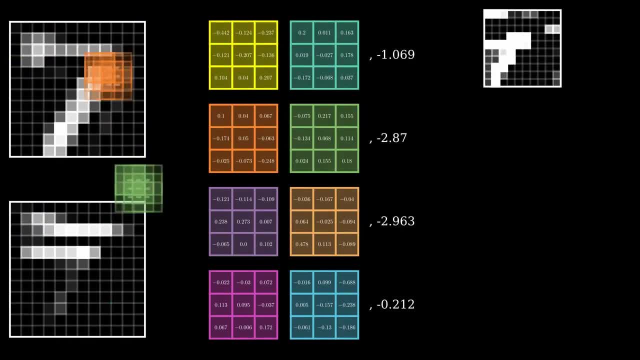 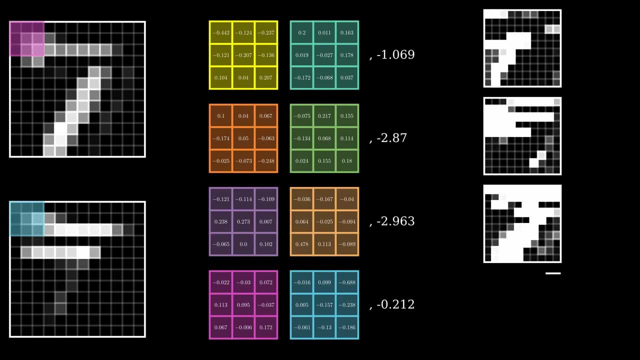 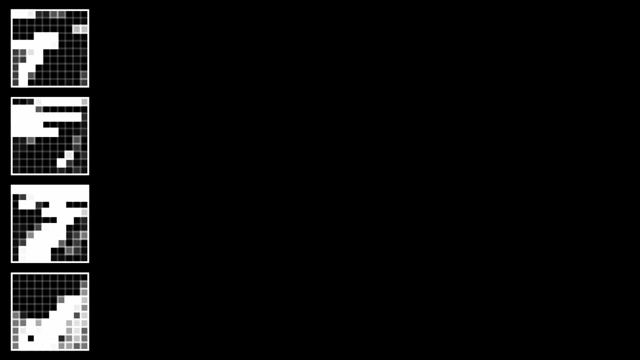 Running the convolution will return four outputs, One for each filter. As you can see, we kind of lose the idea of what the original image was. From this point on, it's hard to decode what is actually going on. But let's continue to the last max pooling. We'll do exactly as we did earlier. 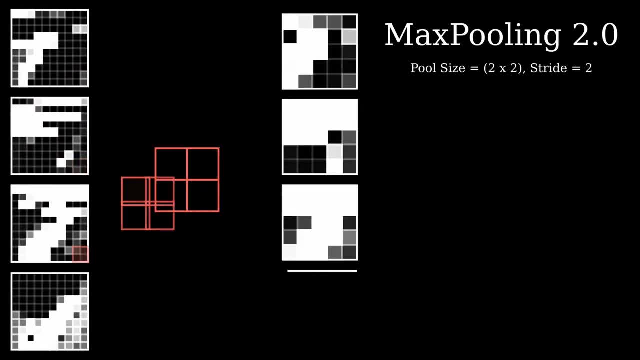 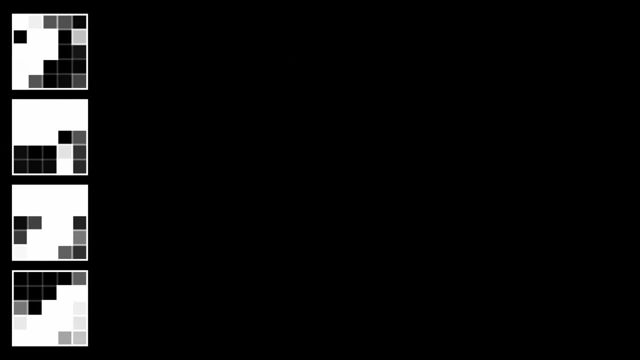 Since there are four channels, we'll output four channels. What we extract is the most activated pixel values from the first convolution. Since we have four channels, we'll output four channels. It will ask: we have programs with different parameters to run in a different method available. 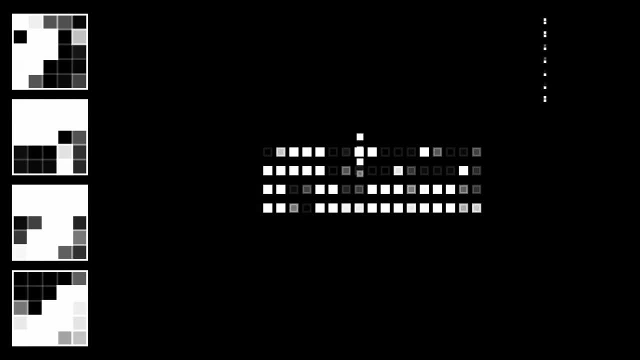 We'll then take these four matrices and flatten them out so that we separate each and every pixel. We went from four matrices that were 5 by 5 to one flat layer with 100 nodes. To make the visualization easier, we'll shrink the nodes so that we only see the first, 5 and 5 last nodes. 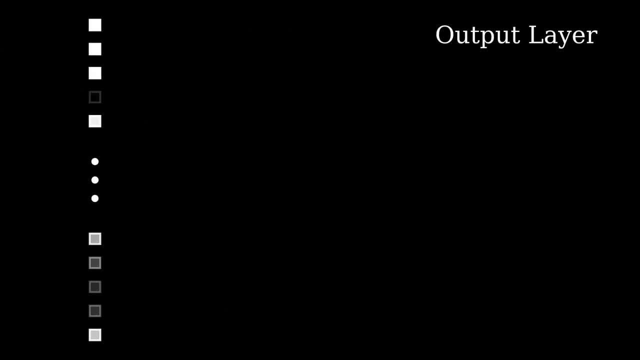 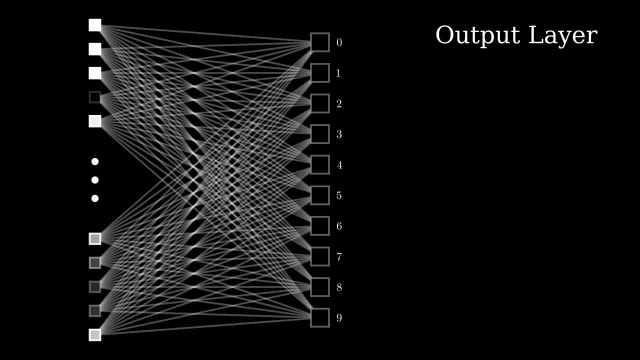 Finally, we have the output layer, where we have three of the 6 nodes and have to change Initially. the entireigare layout has recentшейed to thirty Fr, where we want to output 1 out of 10 different predictions. This is a fully connected dense layer.